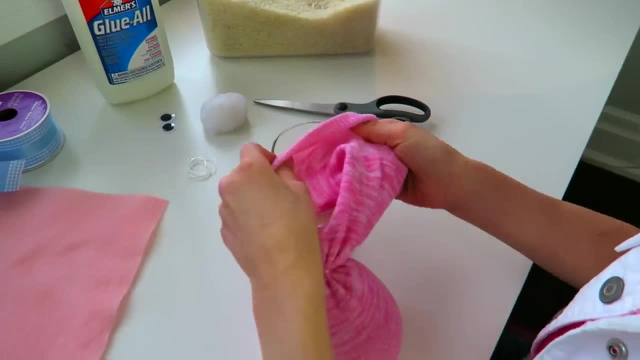 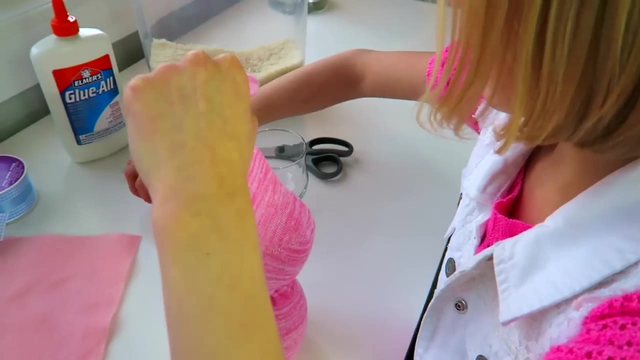 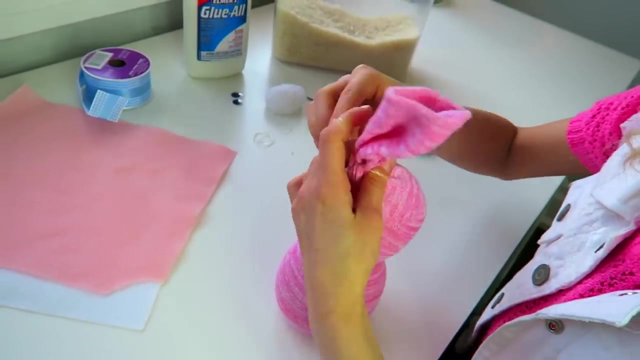 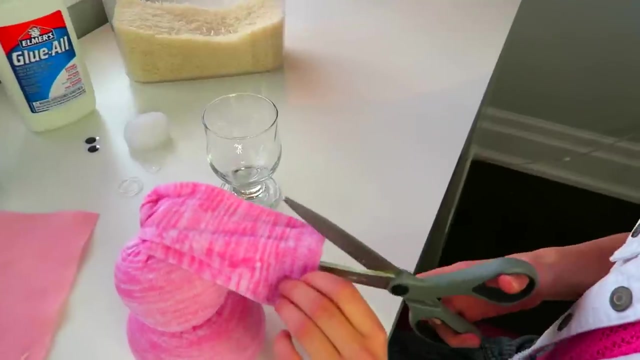 Then you put more rice to make the head, Then you tie it with an elastic band so it can make the shape of a head like. so This is what I have so far. Now you make the ears, You cut out the ears, just like that. 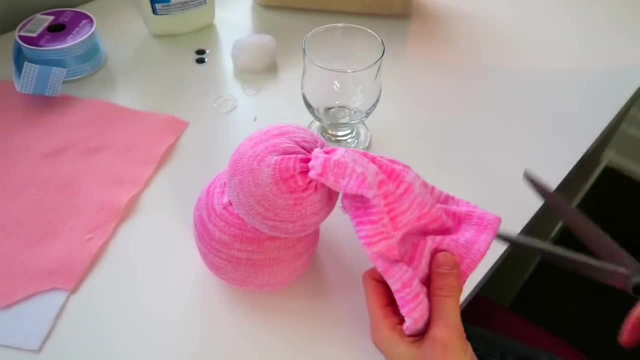 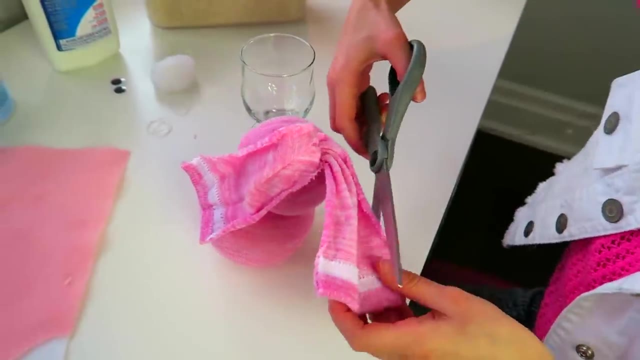 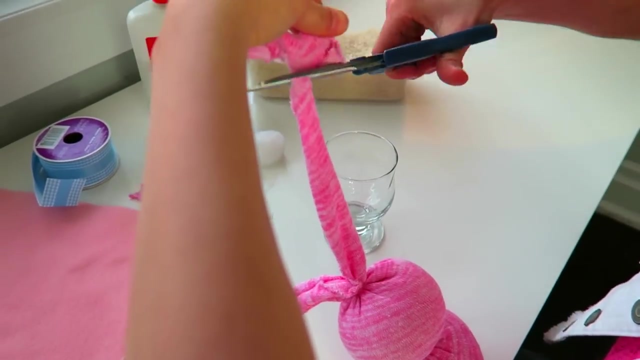 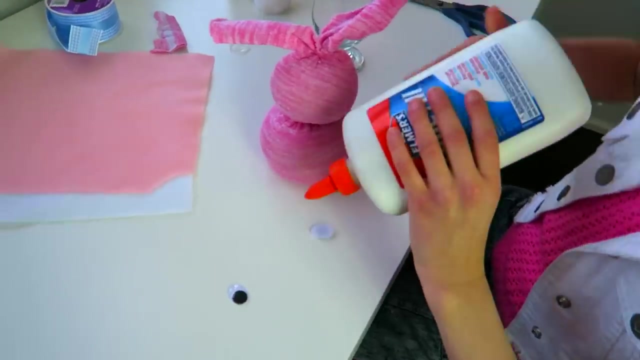 And then the other side. Then you curve them to make it into a kind of bunny shape And you do the other side. This is what I have so far. Now you glue on the two eyeballs Under the eyes. Okay, so when you're done you want to take a little paper towel to make sure you don't. 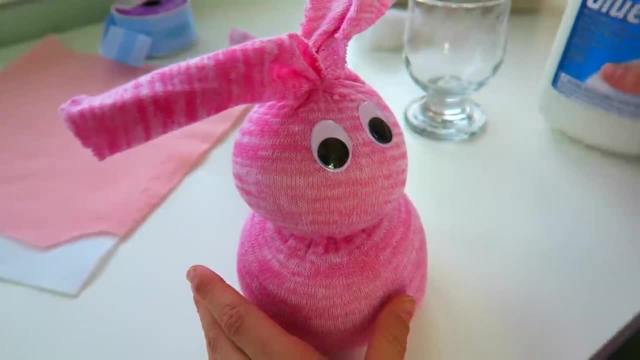 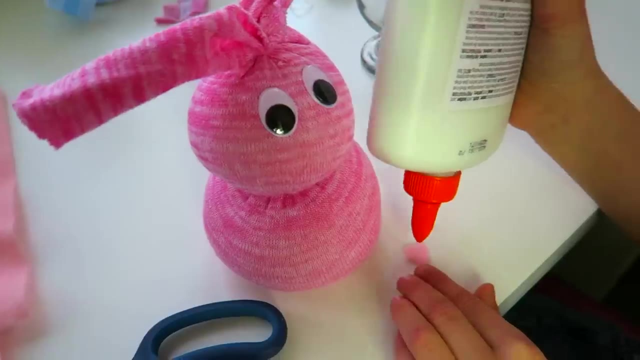 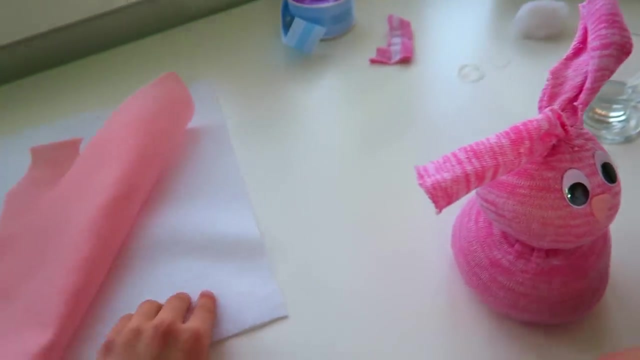 onto the head, take them close to each other, but not too close. then you make the nose. you cut up a small piece of pink of felt and then you make a triangle and then you glue it and stick it on to the head. now you make the teeth, make a kind of pants shape. 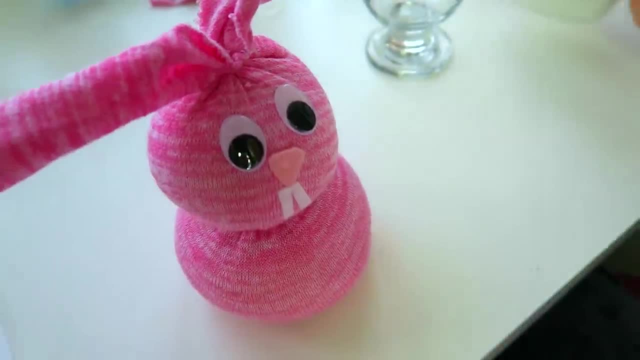 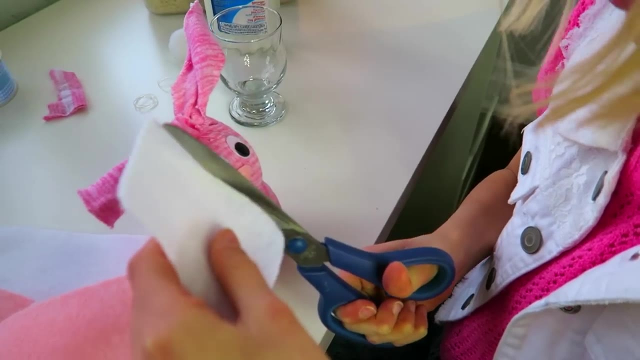 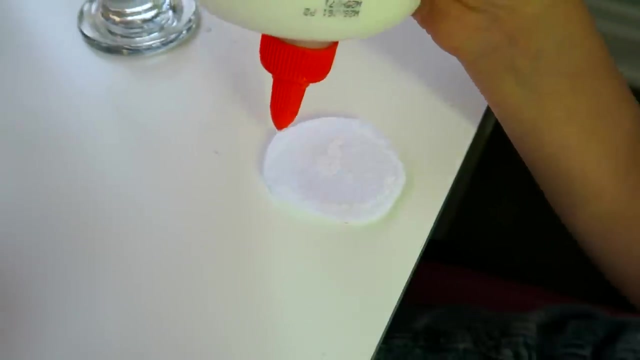 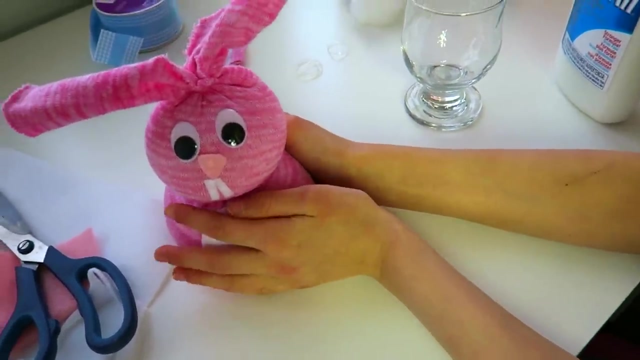 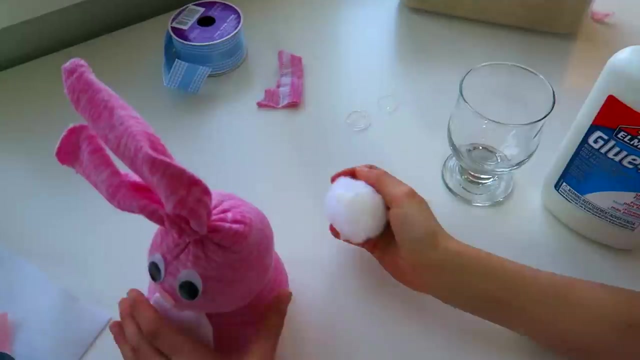 and then stick them on touching the nose. then you make the body well belly. so what you do: cut out a square and then you circle it into a circle with your scissors, then you glue it and then you place it on to your belly. this is what i have so far. next, you take a pom-pom, put glue on it, but 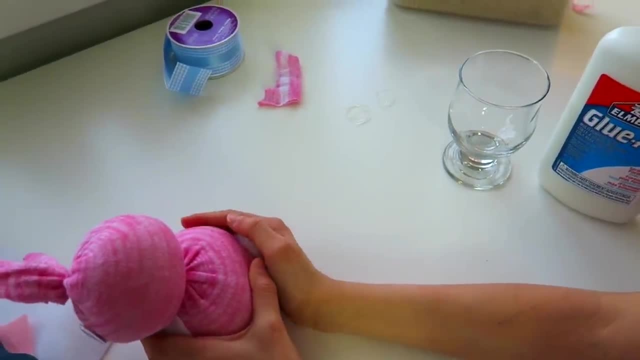 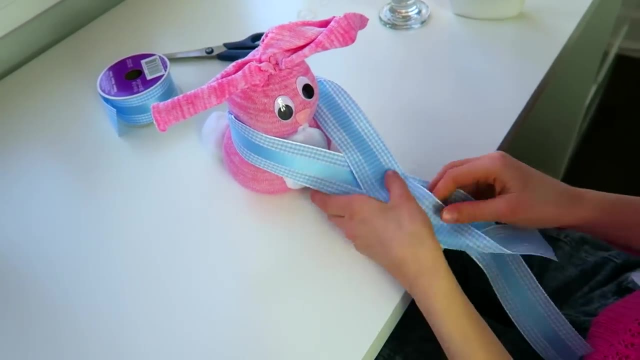 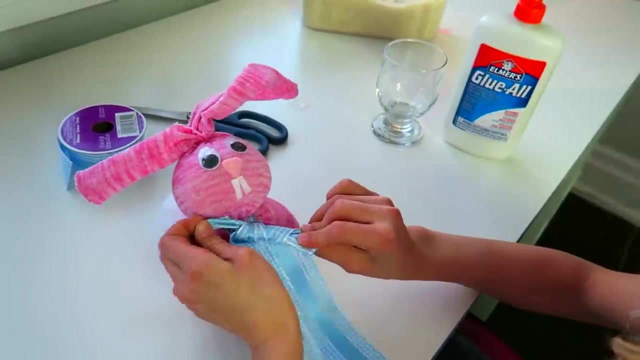 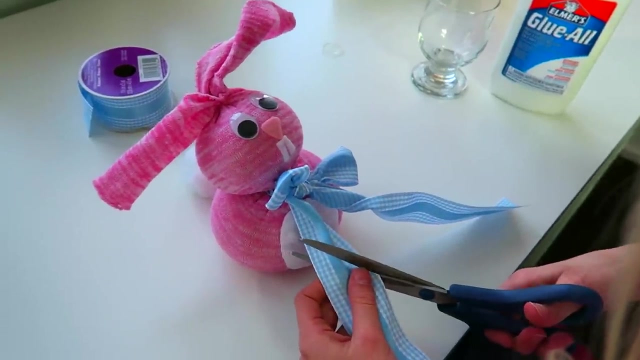 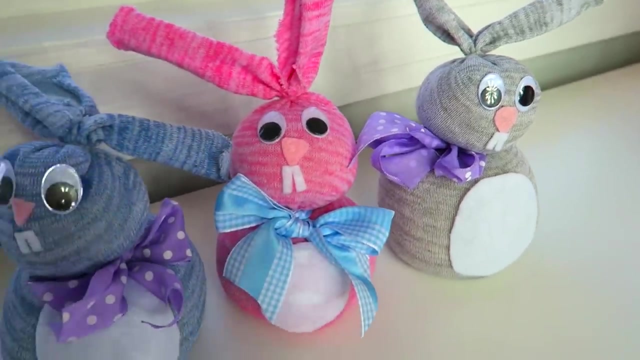 then stick it on right behind it. and the last part: you take a lot of ribbon, you tie it around the bunny's neck and you make a bow like that. then you cut the extra ribbon like in a diagonal shape and you are done. and these are the bunnies i. 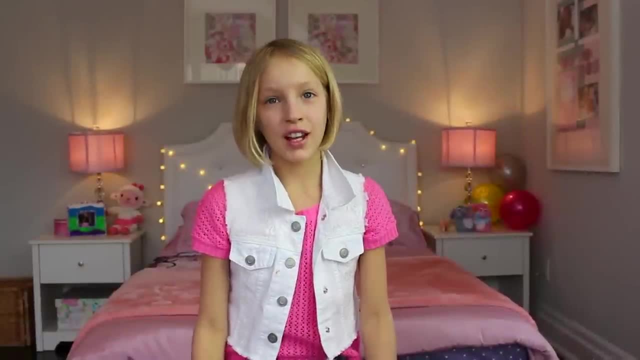 made. okay, guys, i hope you like my video- if you did, give it a big thumbs up- and i'll see you next time. bye.